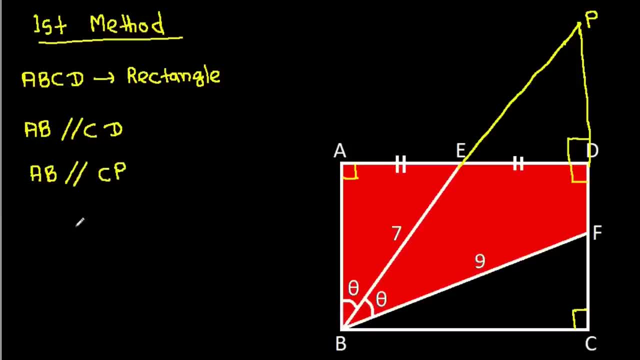 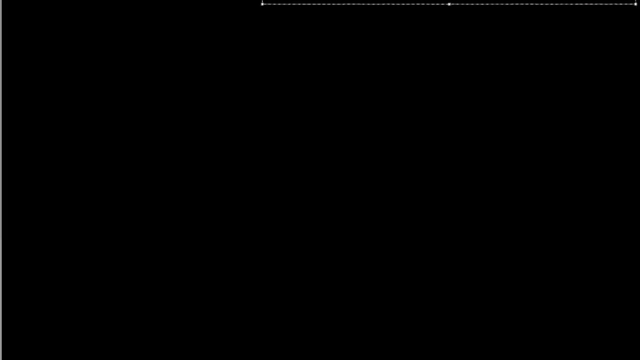 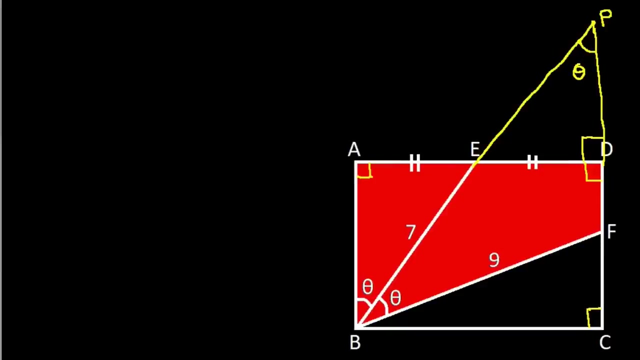 it will be parallel to CP and it is AP and CP and this angle is theta. and we know that AB it is parallel to CP. so this angle, it will be also theta, this angle, it will be theta. and now if we see inter angle ABE and triangle DPE, then we have angle ABE is 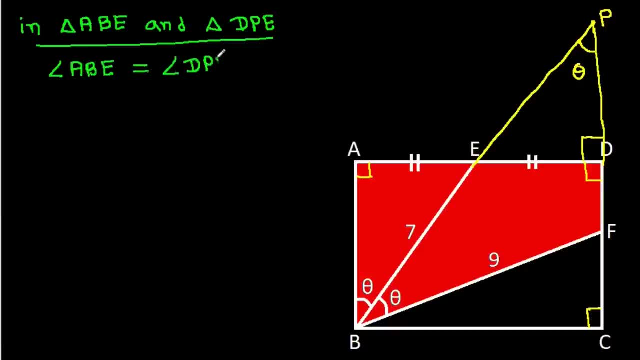 equal to angle DPE, that is, theta angle. Terangle BAE is equal to angle PDE, that is, 90 degree, and AE is equal to DE. it is given So triangle ABE, it will be congruent to triangle DPE, hence BE. it will be equal to PE and BE. 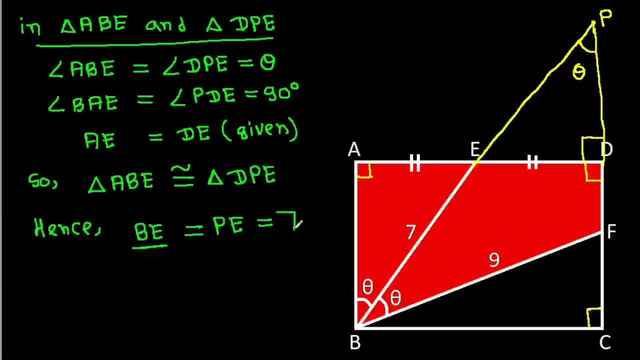 is 7, so PE it will be also 7.. BE it is 7 and also area of ABE it will be equal to area of DPE. suppose x: if this area is x, then this area it will be x. 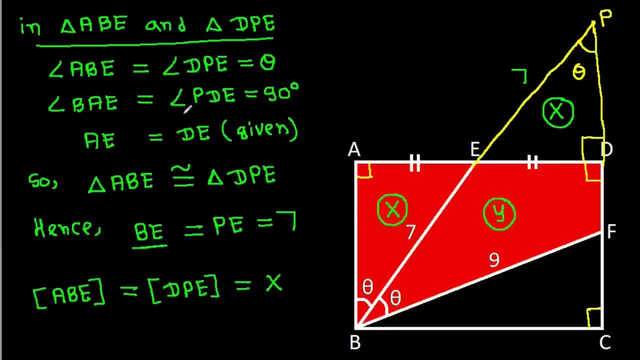 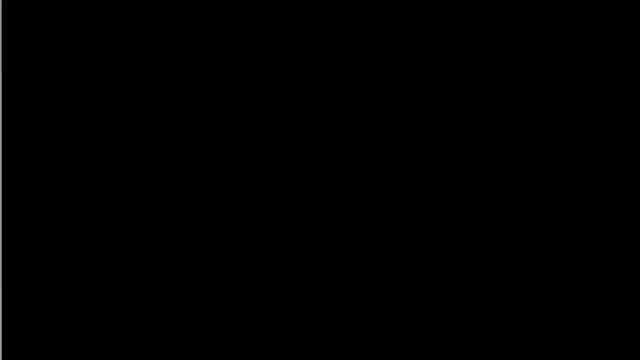 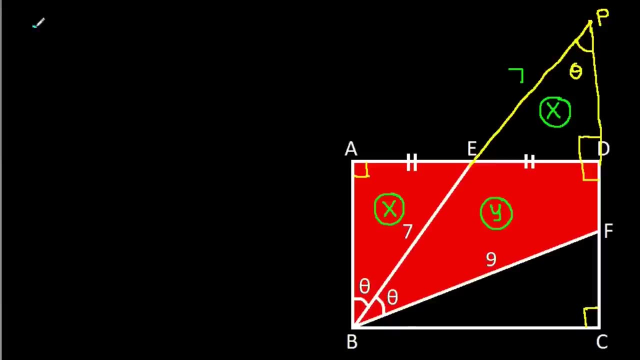 And suppose this area is y, Then here it is shaded area. it is equal to x plus y, x plus y and y plus x plus y, it will be equal to area 7.. So yes, fade area has 2 points. 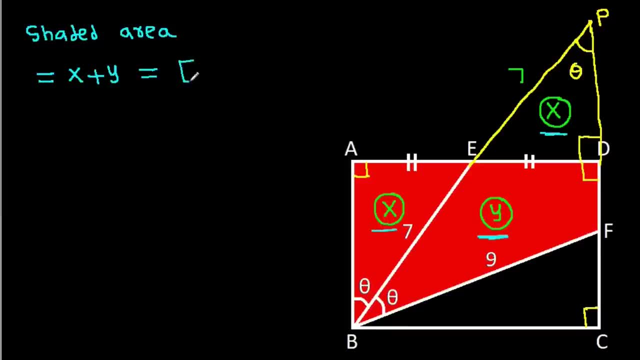 Let's start again. minus y is also area after angle BPF. that means shaded area. it will be equal to area after angle BPF. and now, in angle BPF these two angles are theta. that means it will be isosceles triangle, and this point is E and BE is equal to PE, that is 7 and BF. 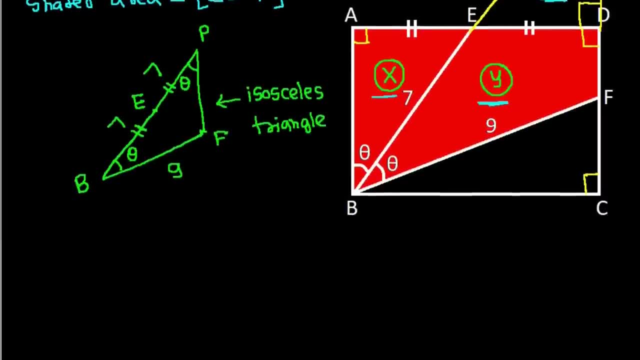 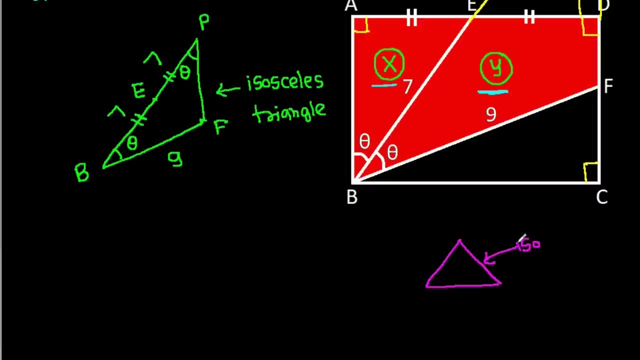 is 9, and in any isosceles triangle, in any isosceles triangle, ABC, if we draw a bisector of BC, then it will be perpendicular to BC. So here, FE, it will be perpendicular to BP. and now in triangle BEF, BF, square, it will 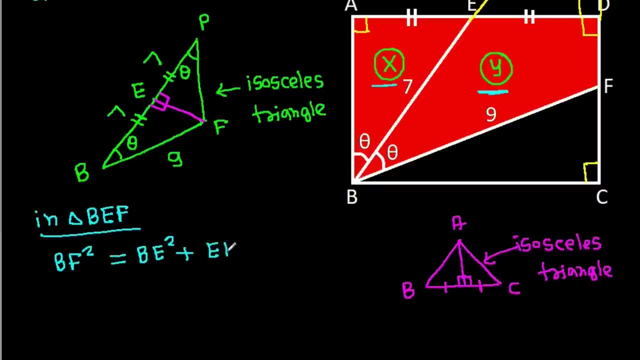 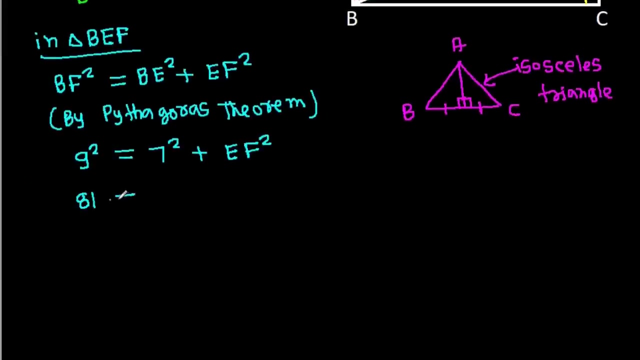 be equal to BE square plus EF square By Pythagoras Theorem and BF is 9 square, it is BE is 7 square plus EF square and it is 81 is equal to 49 plus EF square, So it is 41.. 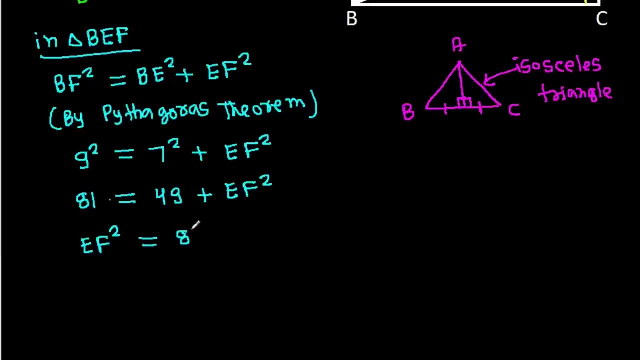 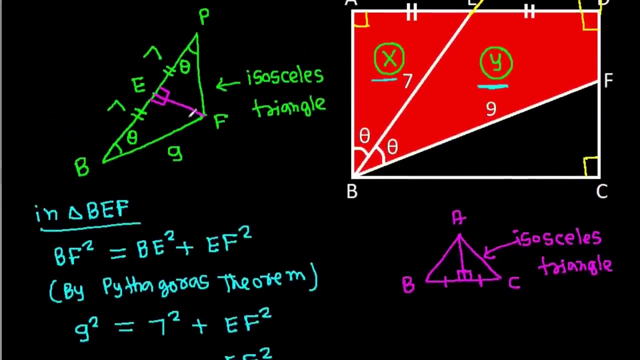 So it is 41.. EF square it will be 81 minus 49,, that will be 32.. So EF it will be S square root of 32, that will be four times S square root of 2.. So EF it is four times S square root of 2.. 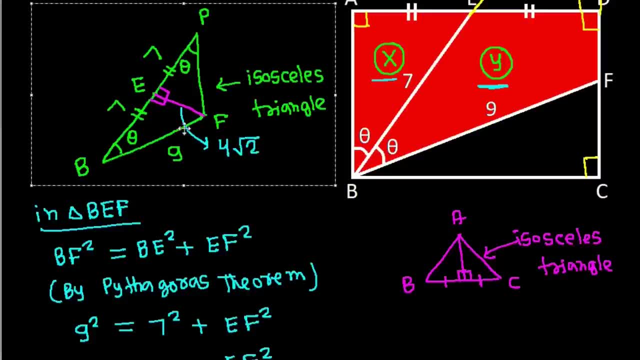 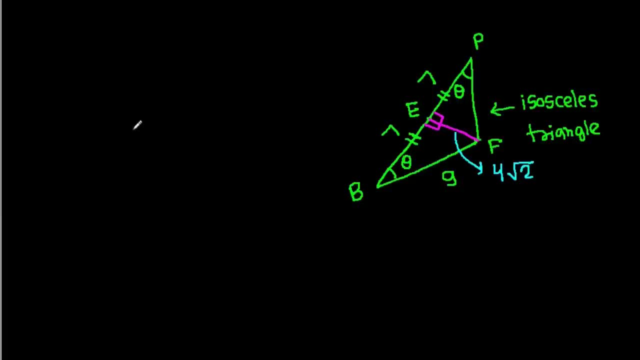 It is not EF, it is 72.. It is 92.. So EF, it is 94.. and now area after angle: BPF it will be 1 by 2 times. base is BP and height is EF, and it is 1 by 2 times. BP is 7 plus 7 times EF is 4 times s square root of 2 and 2 times. 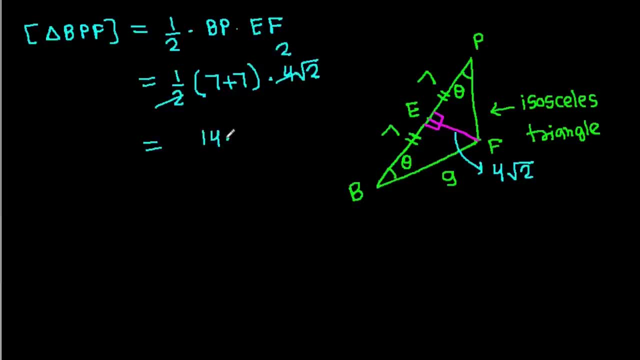 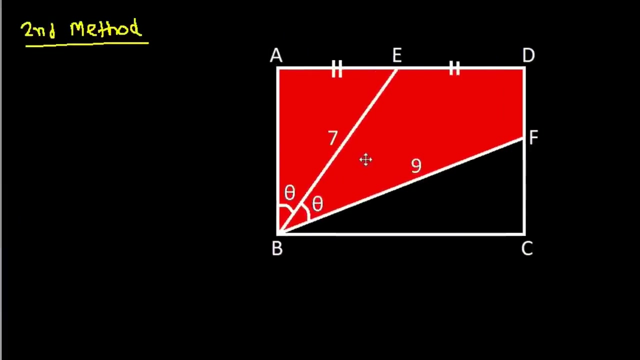 2 is 4, so it is 14 times 2 times s square root of 2. that will be 28 times s square root of 2.. And area of BPF, It is shaded area. that is 28 times a square root of 2. and the second method. we know that. 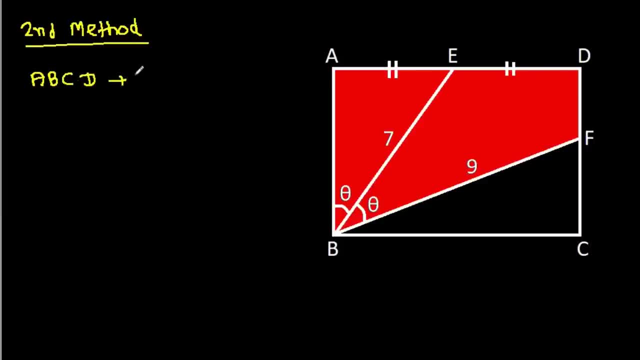 ABCD it is rectangle. so these angles, they will be 90 degree and AB it will be parallel to CD. That means AB it will be parallel to CF And we know that AB and CF are parallel. and this angle it is theta plus theta that will 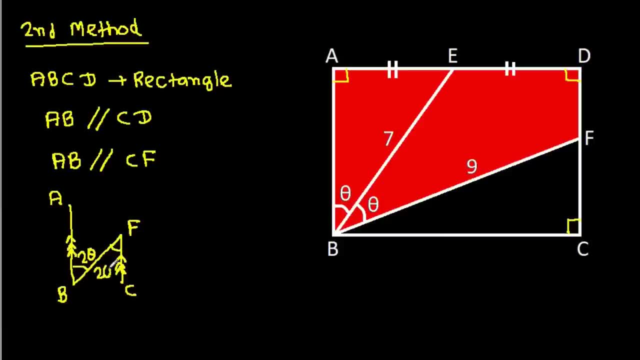 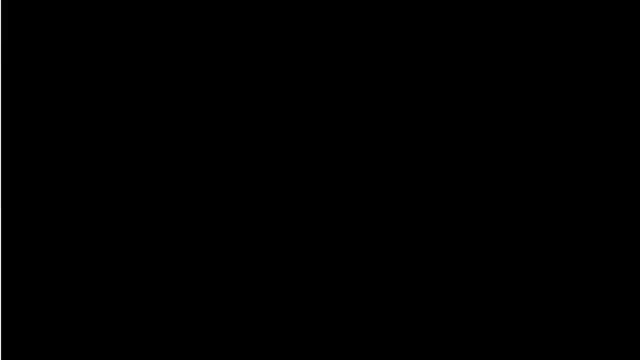 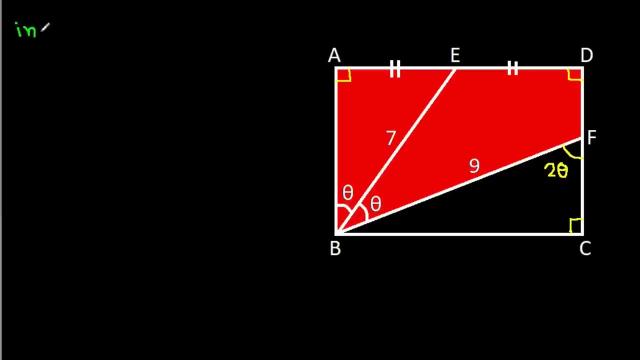 be 2 theta. so this angle, it will be also 2 theta, this angle, it will be 2 theta and this angle, it will be 2 theta. Now, inter-angle ABE: it is ABE. this angle is theta. this angle is 90 degree. 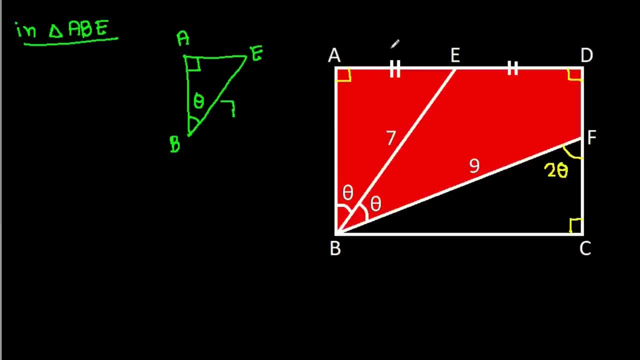 and BE is 7.. and suppose AE is x, then BE it will be also x and BC it will be x plus x, that will be 2x. so we have: AE is x and sine theta it will be AE by BE. so sine theta it is x by 7. and now 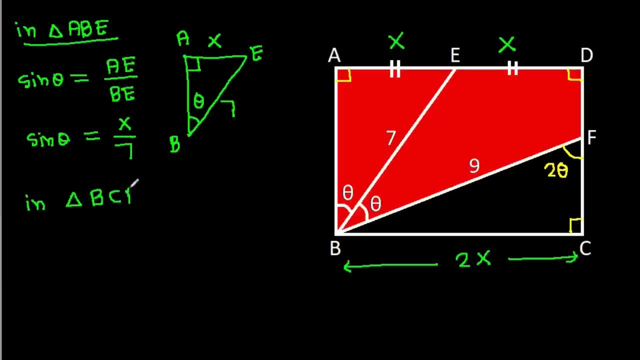 inter-anger BCF. it is BCF. BF is risет 9.. BC is 2x. This angle is 90 degree and this angle is 2 theta, So sine 2 theta it will be BC by BF, And sine 2 theta it is 2 sine theta, cos theta It is equal to. BC is 2x by BF is 9.. 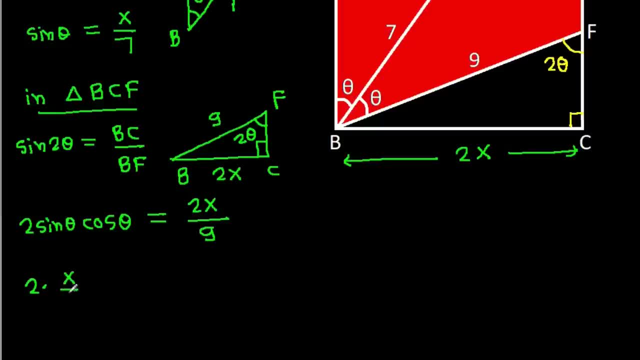 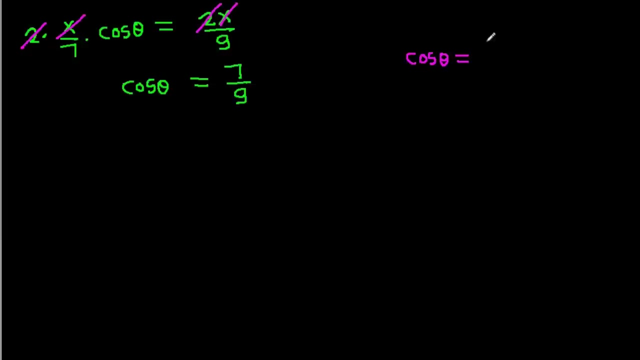 And it is 2 times. sine theta is x by 7 times, cos theta is 2x by 9.. And x will get cancelled, 2 will get cancelled. So we get: cos theta is 7 by 9.. And cos theta it is B by H And sine theta it is P by H, That will be. 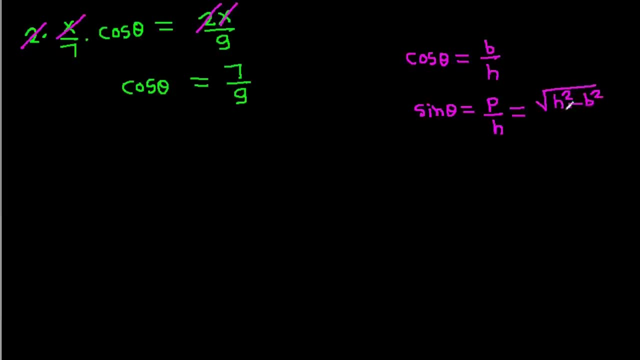 a square root of B by H And sine theta, it is B by H That will be a square root of B by H And sine theta, it is B by H That will be a square root of H square minus B square by H. 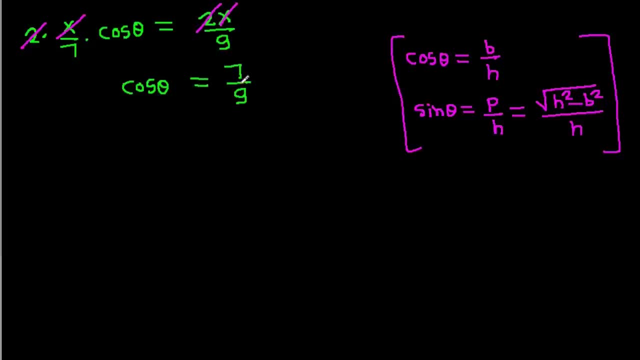 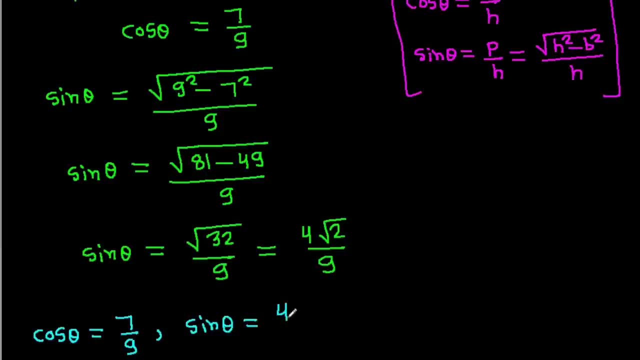 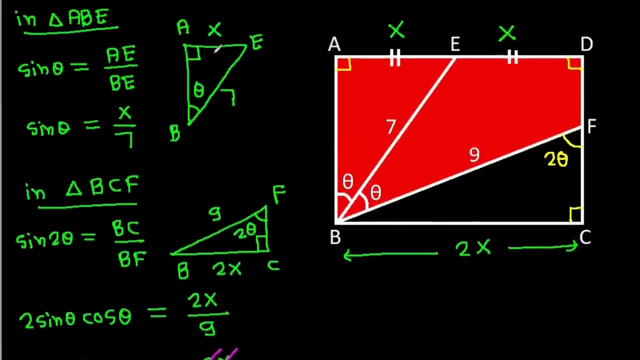 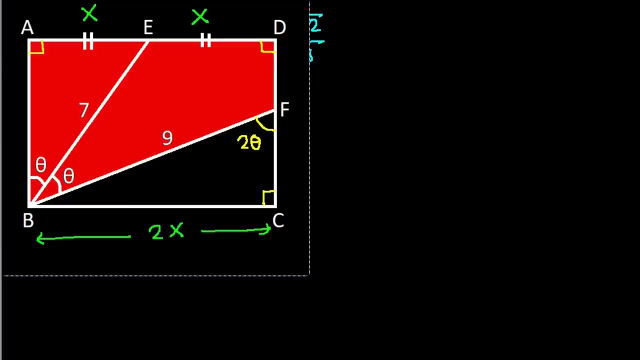 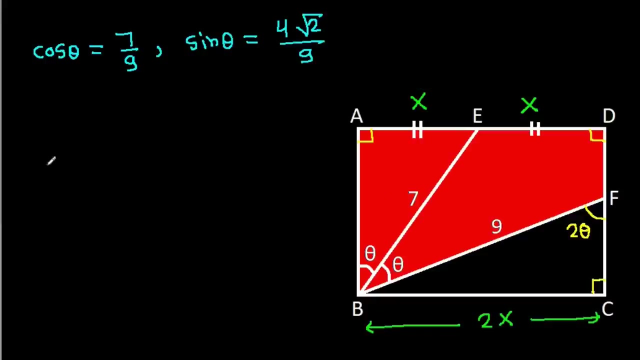 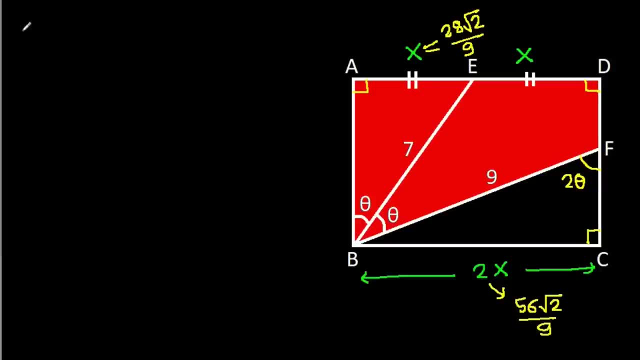 Again, a b it will be be because theta and a, b it is equal to be is 7 and cos theta is 7 by 9.. So we get a- b is 49 by 9.. a- b is 49 by 9.. 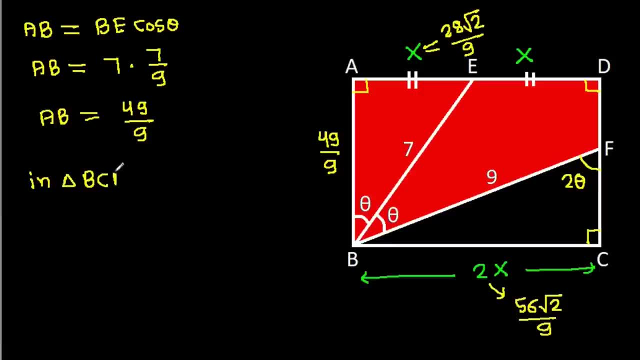 and inter angle bcf. it is bcf. this angle is 90 degree. this angle is 2 theta. bf is 9,, so cf it will be bf cos 2 theta. so cf it is equal to bf is 9, and cos 2 theta it is 2 cos. 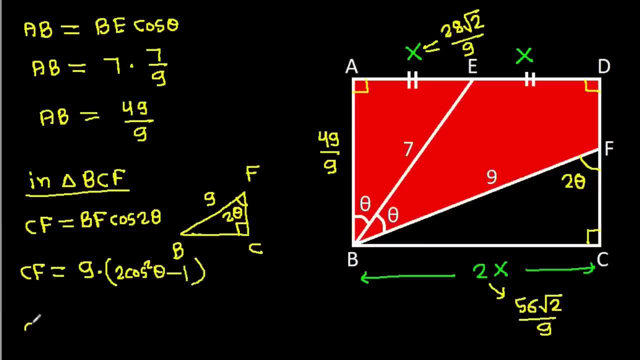 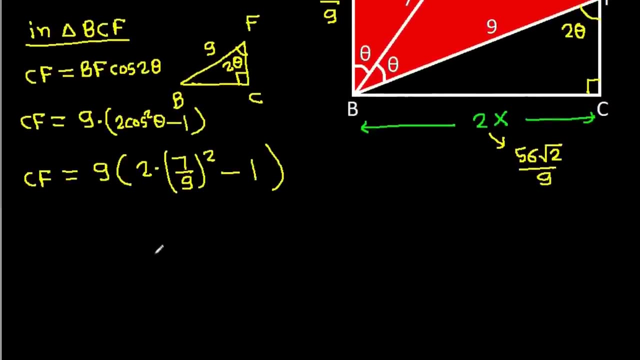 square theta minus 1,, so cf it is 9 times 2, and cos theta is 7 by 9, square minus 1,, so cf it is 9 times 2 times 49 by 81 minus 1, and cf is 9 times 2 times 49 is 98. 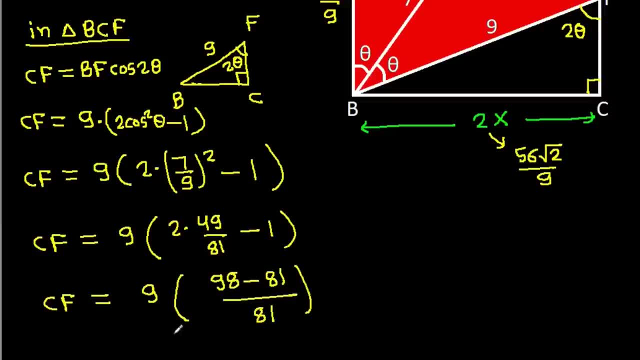 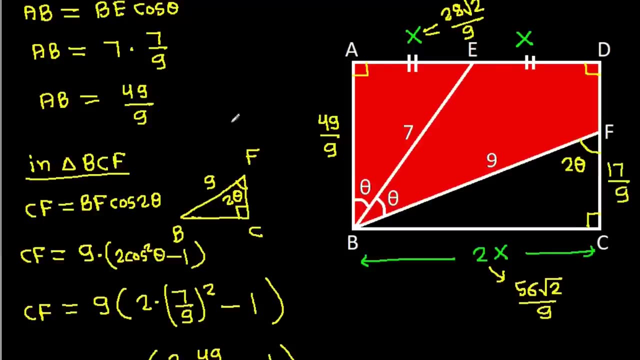 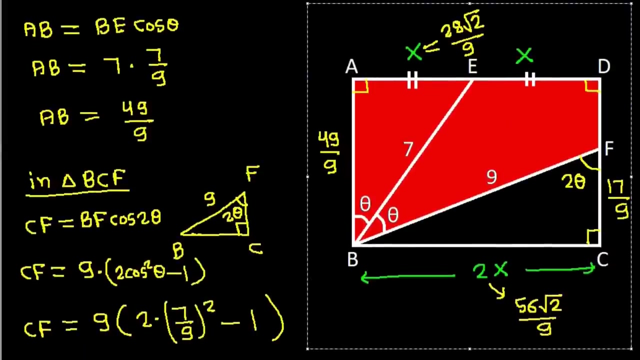 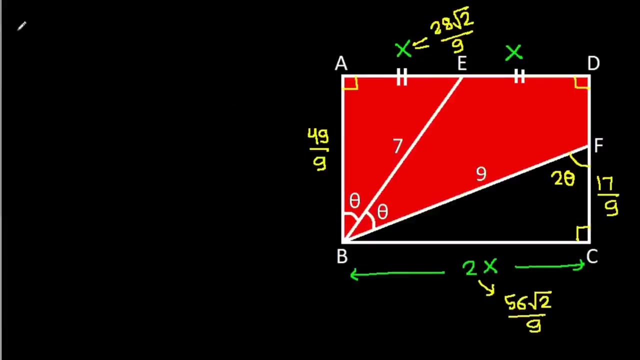 minus 81 by 81, and 9 times 9, is 81,, so it is 17 by 9,. cf is 17 by 9, and now ab, it will be equal to cd, and ab is 49 by 9, and cd is cf plus df, it is 49 by 9, and cf is 17 by 9. minus df, it is 49 by 9,. 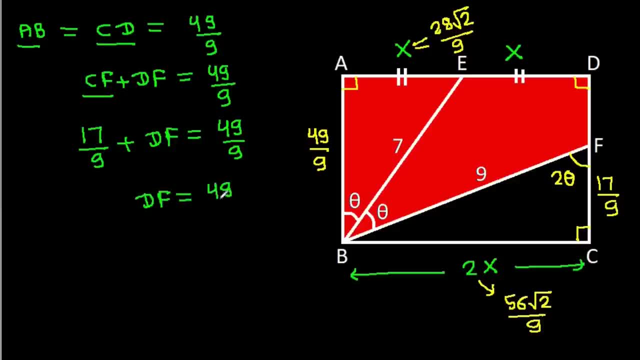 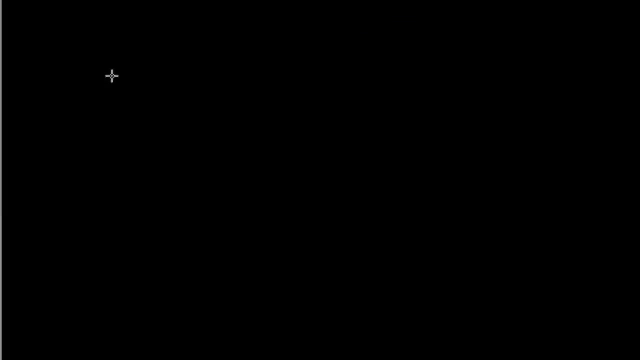 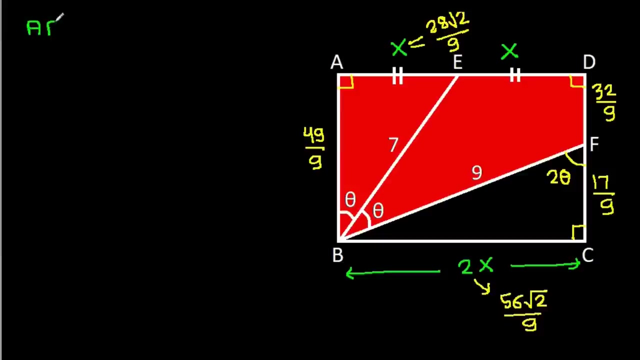 so df it will be 49 by 9 minus 17 by 9,, so df it will be 32 by 9, bf it is 32 by 9, and now abfd it is trapezium. 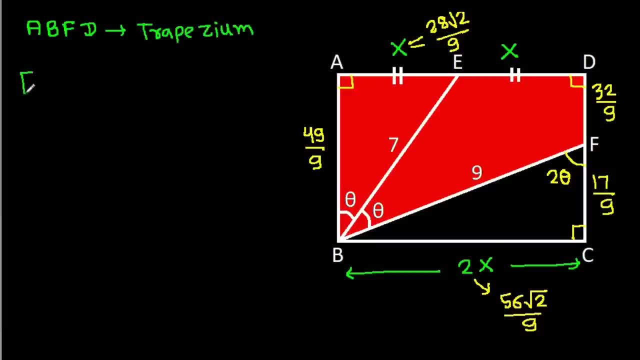 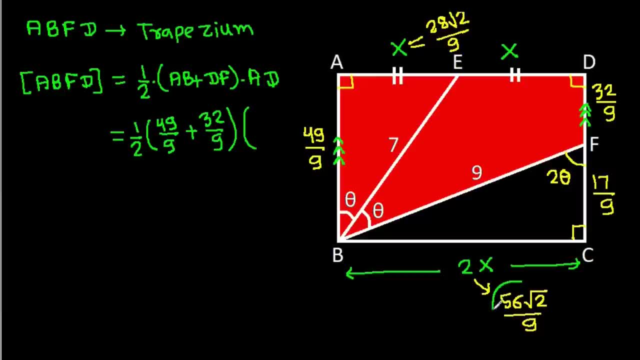 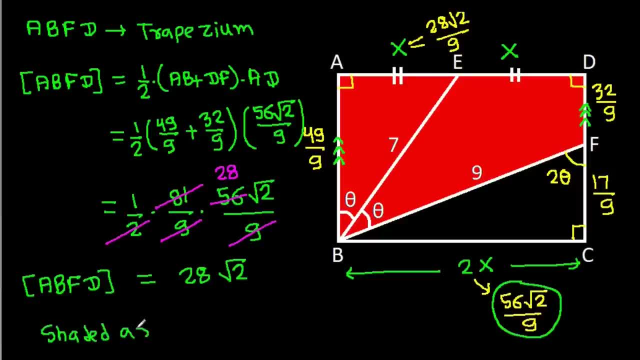 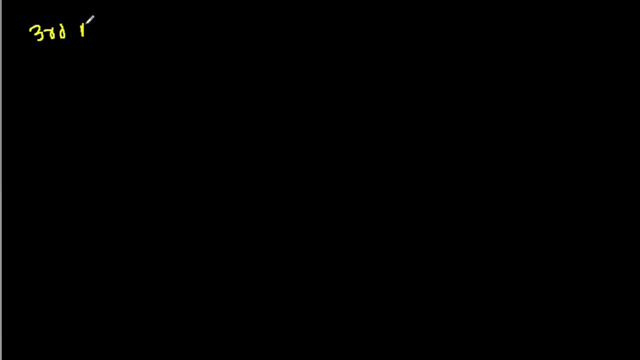 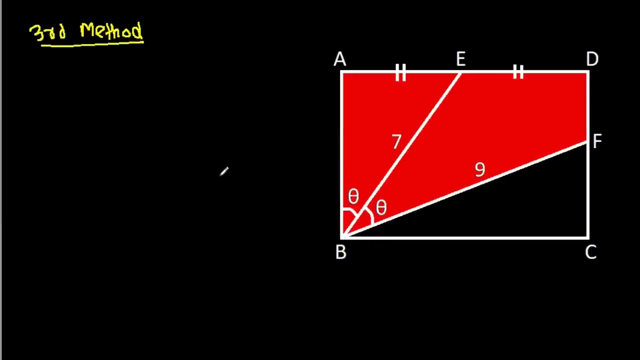 and this is shaded area. so it is 28 times a square root of 2, and now the third method from point E. if we draw a point E, if we draw a point E perpendicular on bf, then we know that abcd is rectangle. 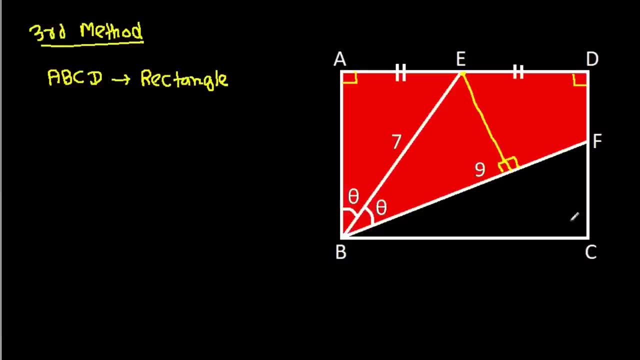 that means these angles are 90 degree. and now in triangle a, b, e and triangle- suppose this point is b- triangle, p, b, e, we have angle a, b, e is equal to angle. 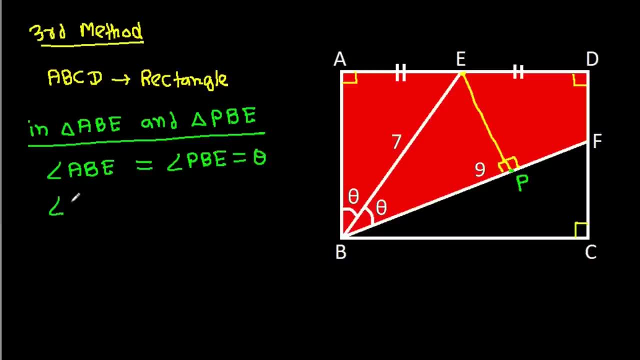 p b e, that is theta angle b a e is equal to angle b b e, that is 90 degree, and b? e is common, that is 7,. so triangle a- b e. 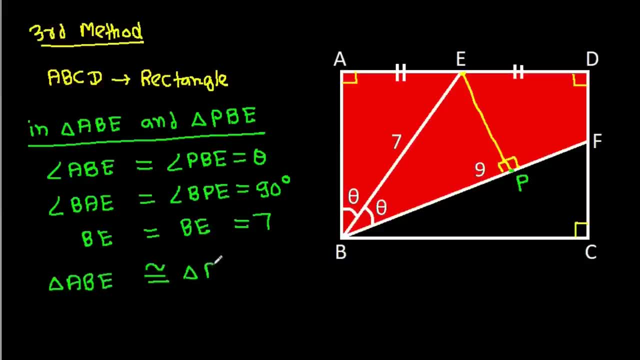 it will be congruent to triangle p b e. that means ab. it will be equal to p b e. and suppose it is y. ab is y and p b is y. 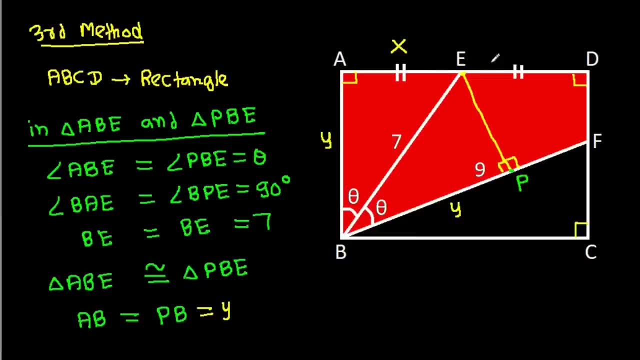 and suppose a e is x, then d e it will be x and b c it will be 2x and a, b is y, so c, d it will be also. 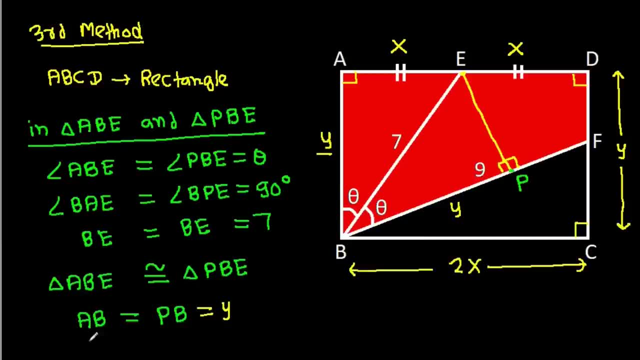 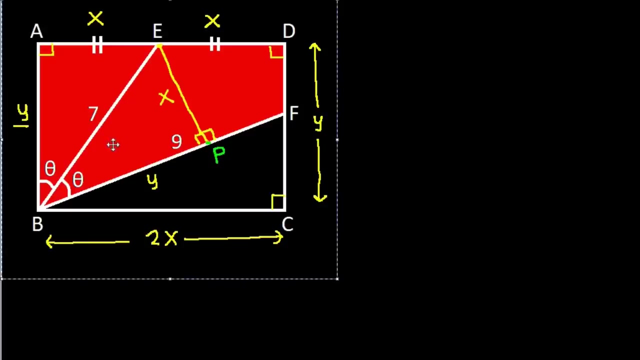 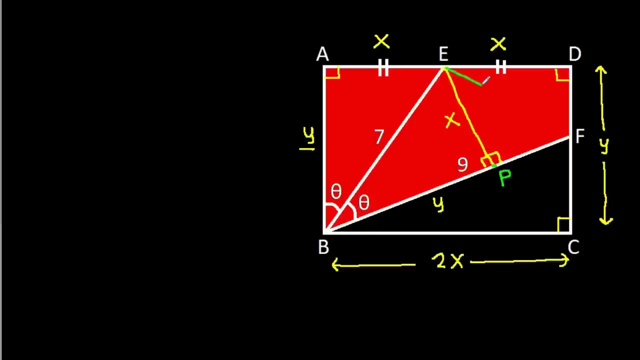 y and also a e, it will be equal to p? e, and a? e is x, so p? e it will be x. and now, if we join e f, then 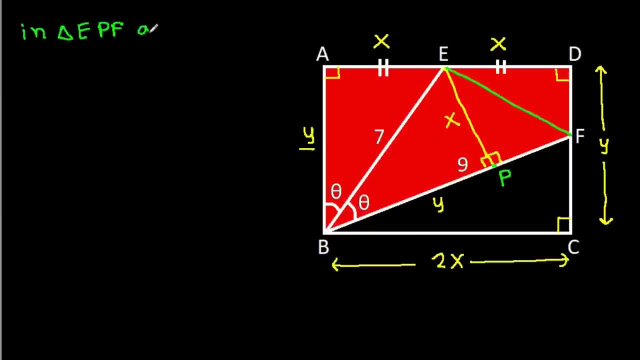 in triangle e p- f and triangle e d- f we have e p is equal to e d, that is x and e f is common and angle e p- f. 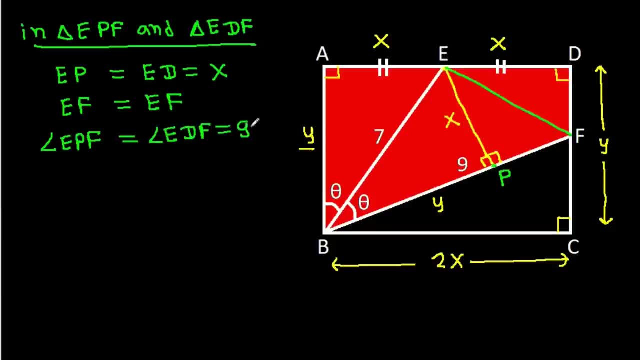 is equal to angle e d f, that is 90 degree. so triangle e p f it will be congruent to triangle e d f, hence p f it will be equal to. 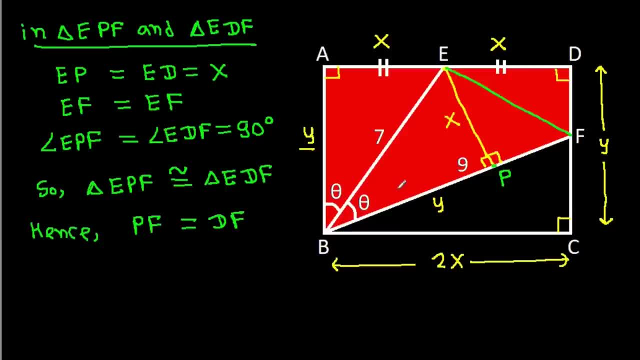 d f and we have b p is y and b f is 9, so p f it will be b f minus b p and b f. 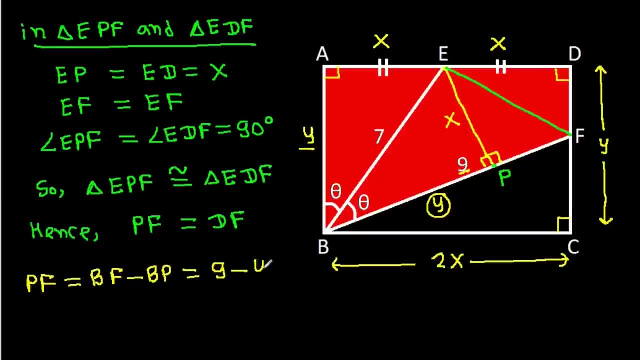 is 9, minus b. p is y, so p f it is 9 minus y, so d f it is equal to p f. that will be 9 minus. 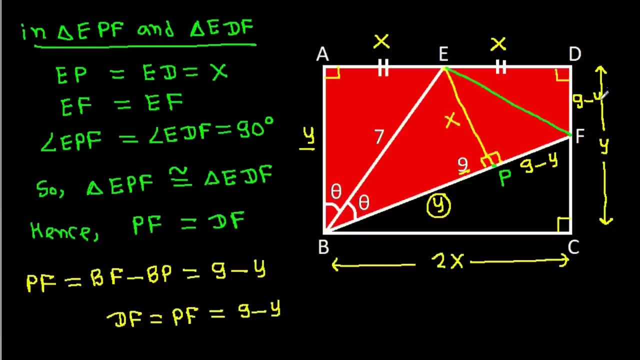 y d f is 9,. minus y and c f, it will be c d minus d f and c d is. y minus d f is 9,. 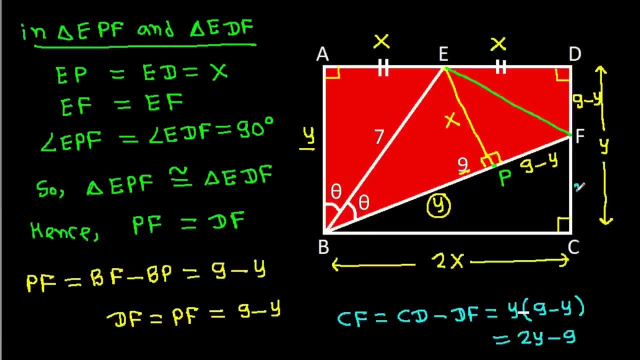 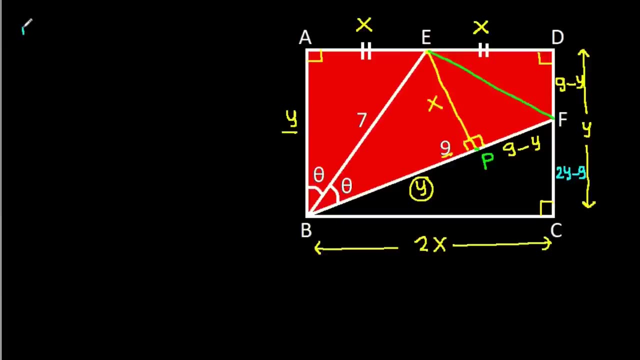 minus y and it is 2y minus 9,. so c f it is 9 minus y and c f is 9, minus y minus 2y. 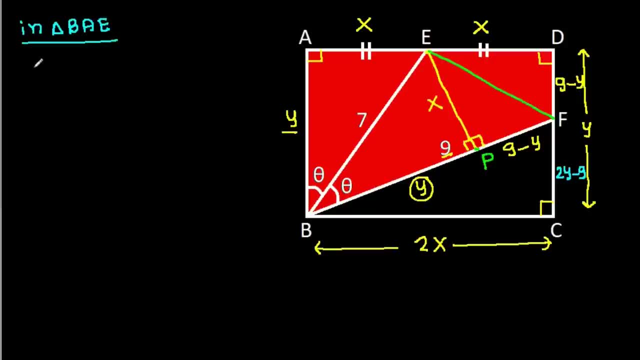 minus y is 1, minus y 1, minus 2y. minus 2y minus 1,. minus 2y minus 2y is c f. 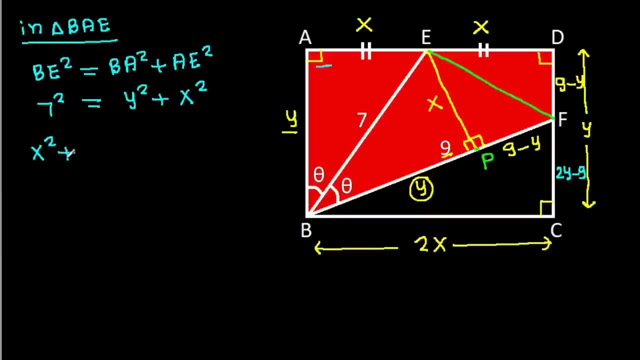 is so we get x square plus y. square is 49 and inter angle b c, f, b f square, it will be b? c square plus c f square and it is 9 square is equal to 2 x square plus c f is 2 y minus 9 square, so 81. 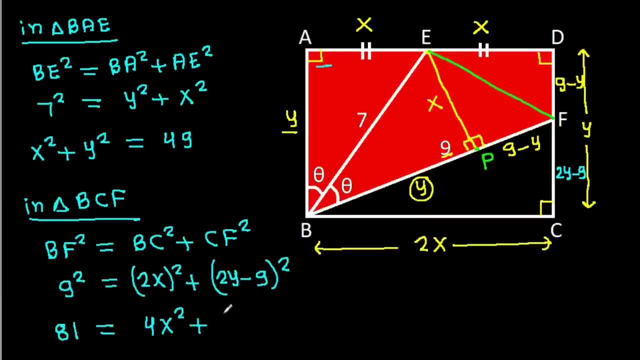 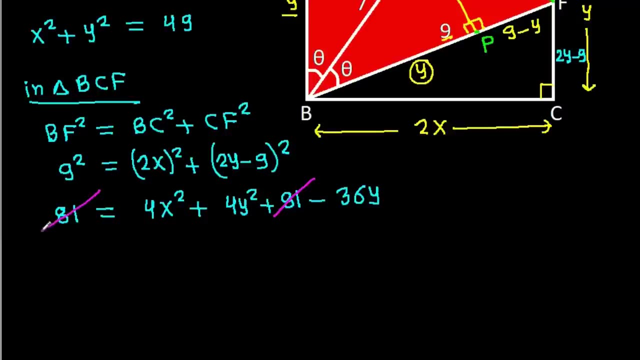 is equal to 4 x square plus this will be 4 y square plus 81 minus 36 y, and 81 will get cancelled. so it is 0 is equal to 4 times x square plus y square is 49 minus 36 y, so 36 y it is 4 times 49 and 4 times 9 is 36. 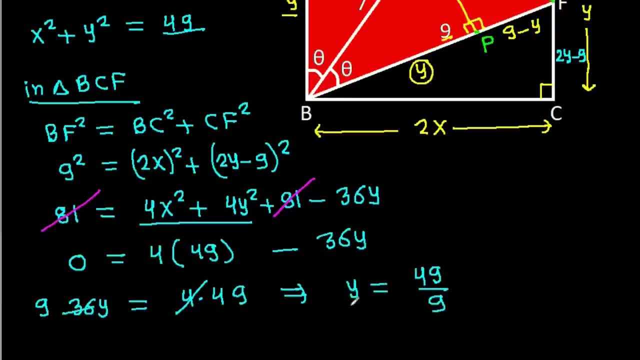 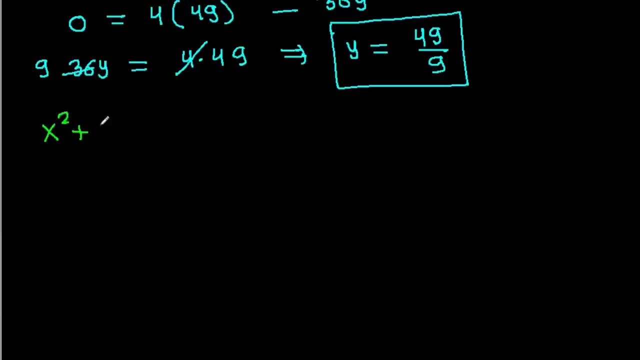 so y it will be 49 by 9 and we have x square plus y square is 49. we have x square plus y square is 49 and x square plus 49 by 9 square it is 49 is 7 square. so x square it will be 7 square minus 49 by 9 square and x square it is 7 plus 49 by 9 times. 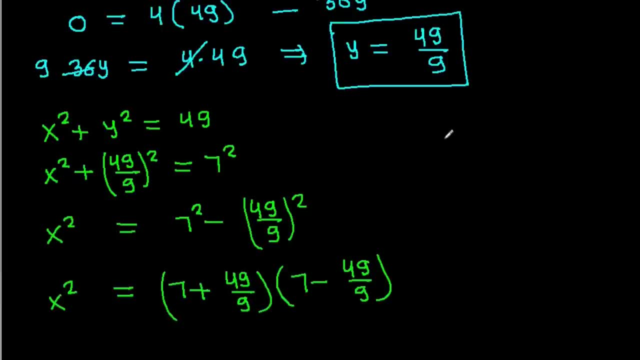 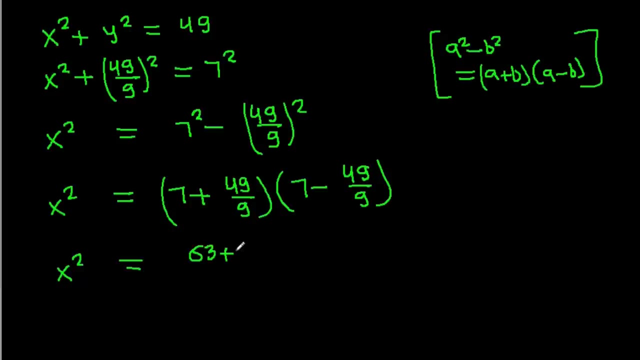 7 minus 49 by 9, because a square minus b square, it is a plus b times a minus b. so x sqa, so x sqa. it is 63 plus 49 by 9 times 63 minus 49 by 9 and x square. 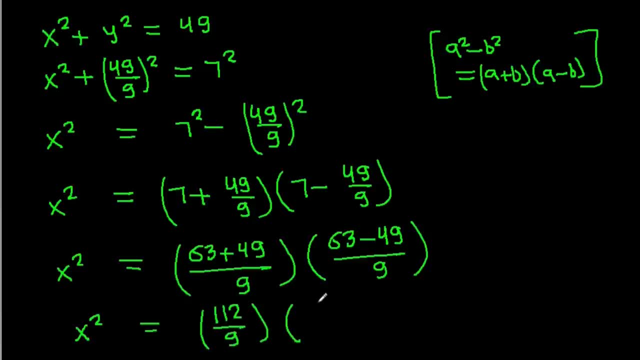 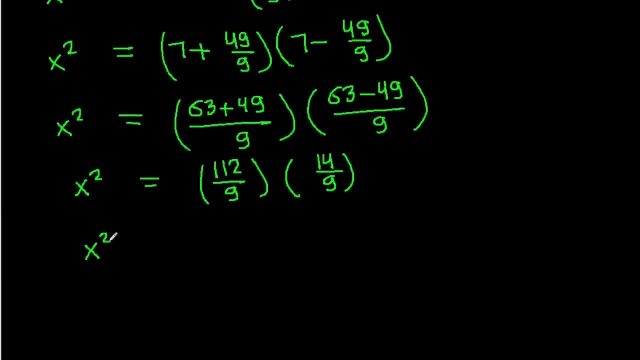 it is 63 minus 49 by 9 x 63 minus 49, it is 123 by 9 times 14, it is 123 by 9 times 14. by 9, it is 123 by 9 times 14 by 9 and x square, it is 129 and x square is 112 by 9 times 14 by 9. Prime. 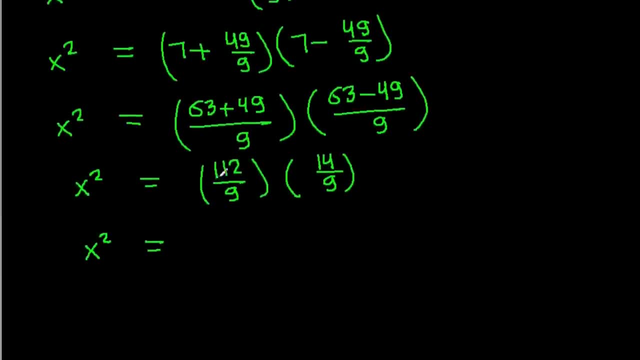 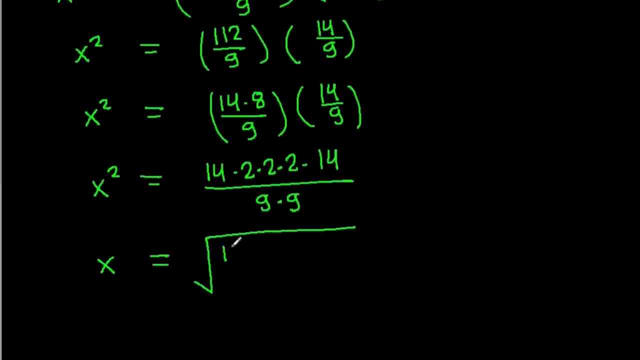 x square, it is equal to 112. it is 14 times 8 by 9 times 14 by 9. and x square, it is 14 times 8, is 2 times 2 times 2 times 14 by 9 times 9. so x will be equal to a square root of 14 times 2 times 2. 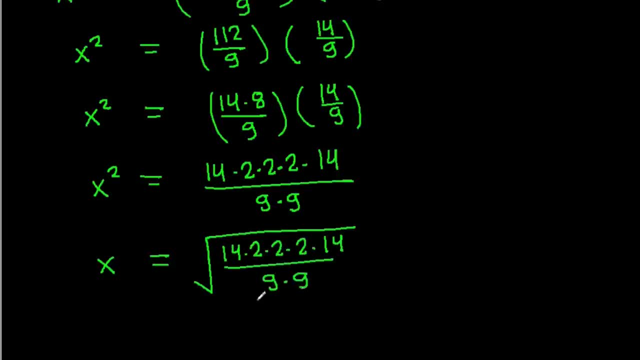 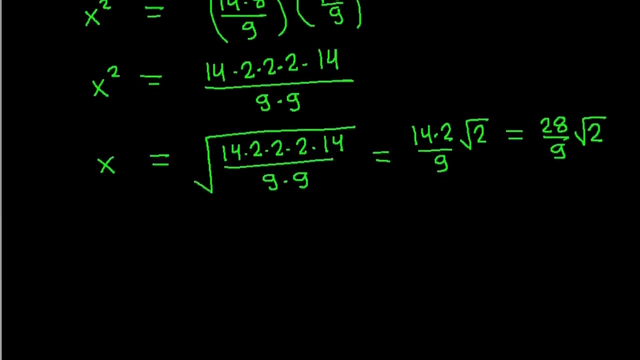 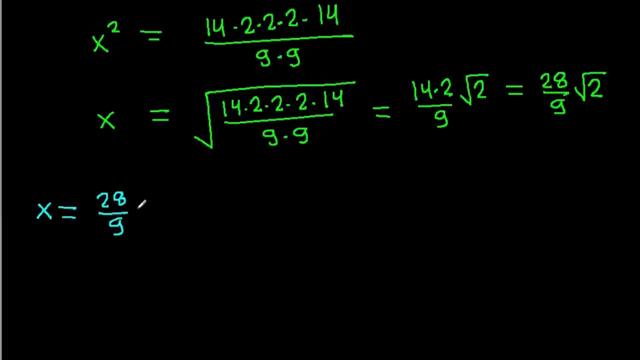 times 2 times 14. by 9 times 9, that will be 14 times 2 by 9 times a square root of 2, and it is 28 by 9 times a square root of 2, so we get: x is 28 by 9 times a square root of 2.